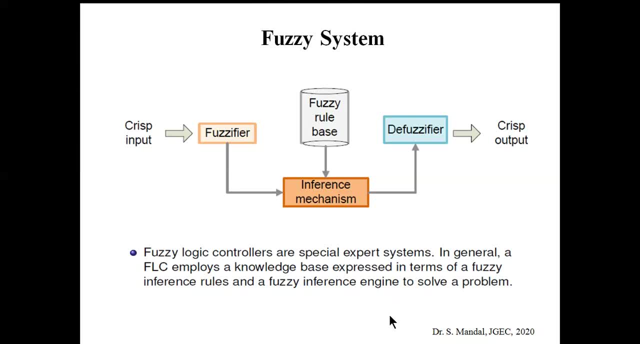 We have already studied it in the earlier class, So now let's revise it. So a fuzzy logic control system: have input, Crisp input and it goes to the fuzzifier and there is fuzzy rule base where different fuzzy rules are already stored there. 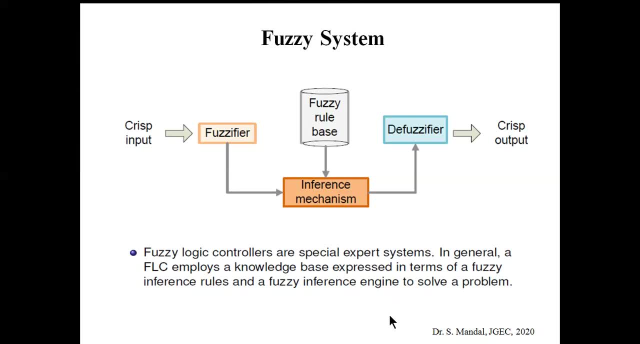 And from there, by using some kind of inference mechanism, we can get the fuzzified output from the inference engine. And now to get the real-life crisp output we need to use de-fuzzifier that de-fuzzify a fuzzified output into the crisp input. 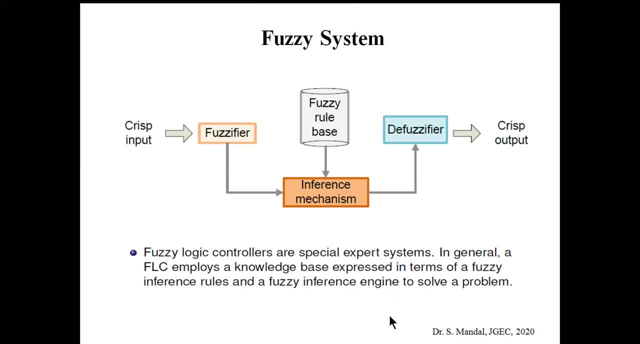 And fuzzy logic controller or fuzzy system is widely popular where precise mathematical formulation is not available to user. So FLC or fuzzy logic controller employs a non-fuzzy logic controller. It employs a knowledge which is expressed in term of fuzzy inference rule And we need to use a fuzzy inference engine to solve a particular real-life problem. 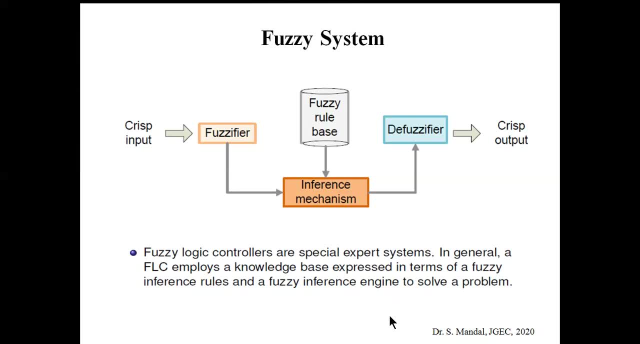 So that is the basically fuzzy system or fuzzy logic controller That should have a input crisp. input and output should be in crisp also. But in between them there is some kind of fuzzifier inference engine and de-fuzzifier to get the crisp output. 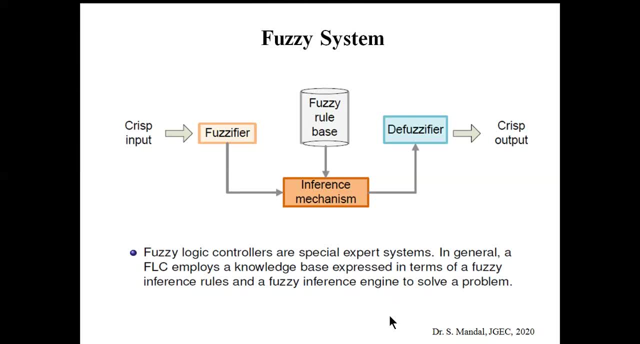 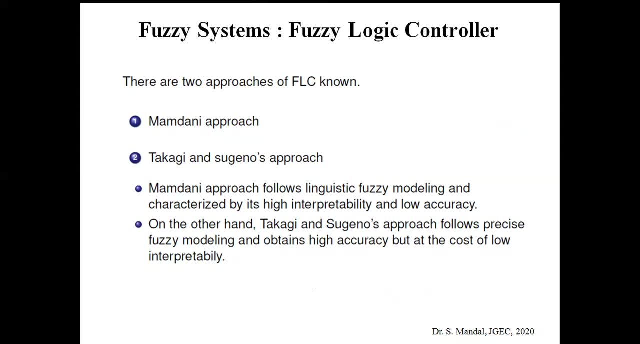 Now in the literature, two approaches are widely popular, very popular. First of all is Mamdani approach and second is the Takagi and Shugano approach In between them. Mamdani approach is very simple and it follows linguistic fuzzy modeling. 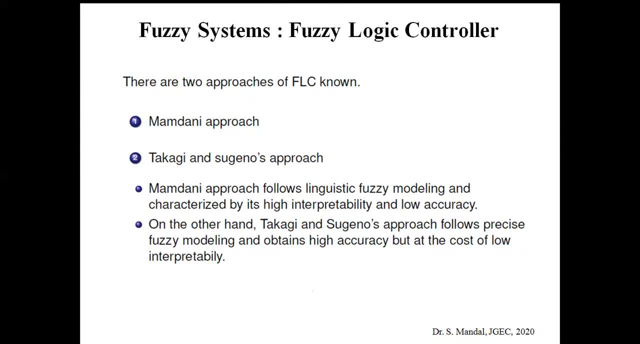 And it is characterized by its high-level analysis. And it is characterized by its high-level analysis And it is characterized by its high-level analysis, But its accuracy is some kind of low, Whereas Takagi and Shugano approach has very high accuracy but it has very low interpretability. 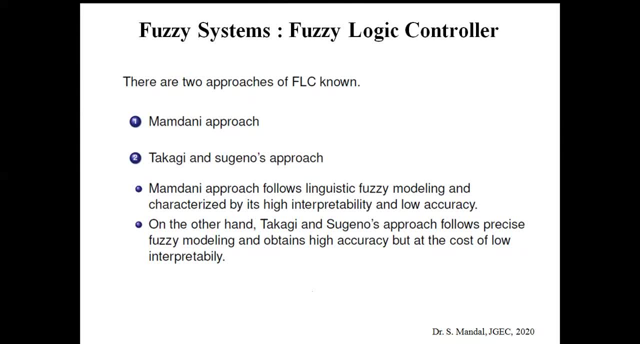 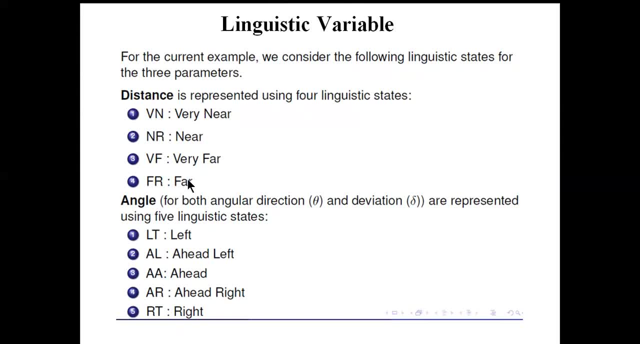 So in this class, basically, we shall discuss about the Mamdani approach: very near, near, very far, far. so very near is defined by sorry, is denoted by vn. near is defined by nr, vf is defined by vf and fr is far. okay, so all these are the linguistic variable and it can. 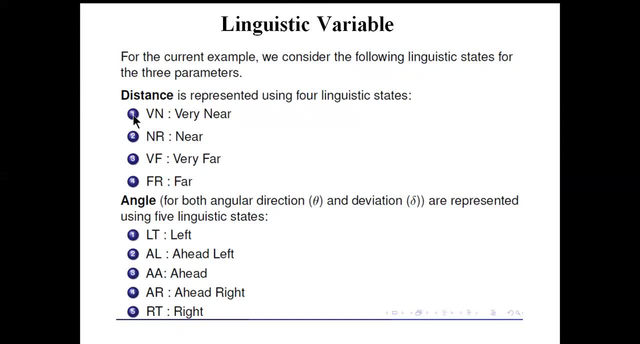 be expressed in term of membership function. similarly, for angle, angle may be angular direction theta and deviation delta. both are angle, so they can be expressed in term of five linguistic state. first of all, left, ahead, left, ahead, ahead, right, right. okay, so left is denoted by lt, ahead, left is denoted by al, ahead is denoted by aa, ahead, right, ar and right is denoted by rt. 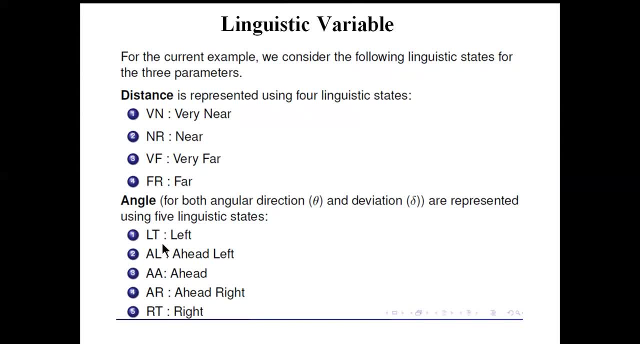 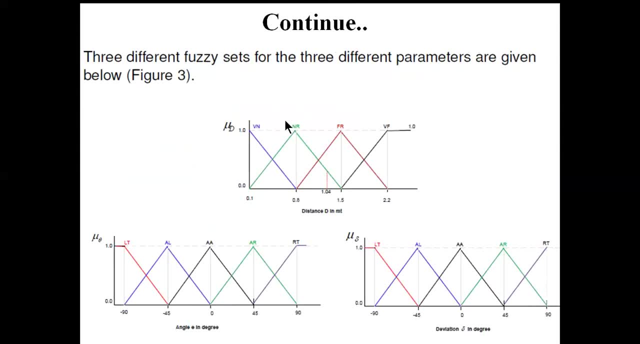 okay, so obviously these angle or linguistics, five linguistic state, are also expressed in term of membership function. okay, so here you can see the corresponding membership function, like you can see that, uh, you, this one for the d distance membership function for the distance. this one for blue color denote. 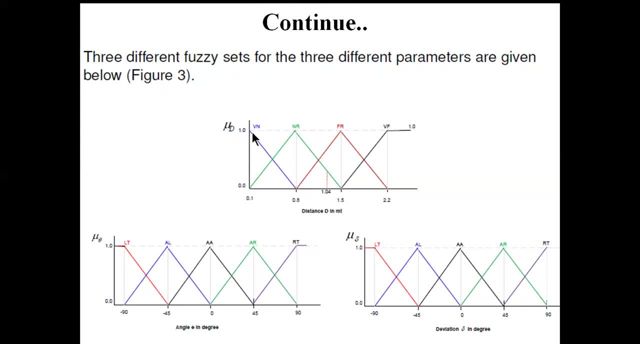 the very membership function for the vn, or very near linguistic variable. okay, here you can see that, uh, the variable from range from 0.1 to 2.2. okay, so when the d is 0.1, obviously the membership function for vn- that means object- is very near. so membership function is one and as we as the value. 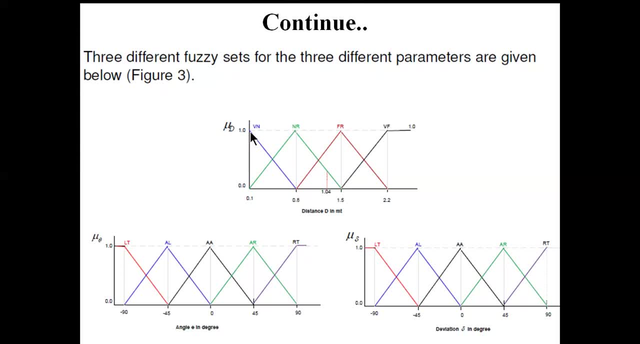 of d is gradually increasing. obviously, very near membership function of the membership function for the very near will be gradually decrease because object is gradually far away, going far away from the robot. okay, so that's why it is it has. it is decreasing linearly like this way. So, similarly, this one is the an r near, this one is 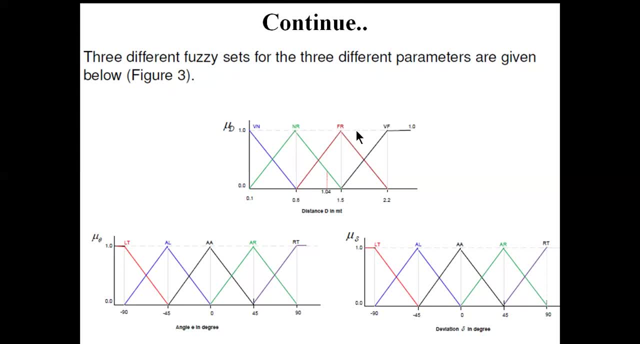 the point five meter, that the maximum value, or that can be called as the near. so that's why the corresponding membership value is one. like this way, the corresponding membership value can be defined by the user or the systems. okay, similarly, you can see that theta value of the theta can be: 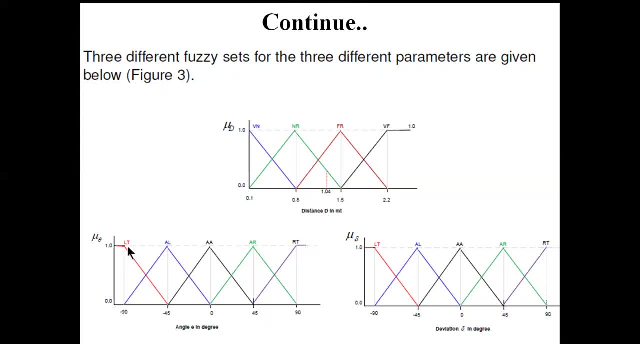 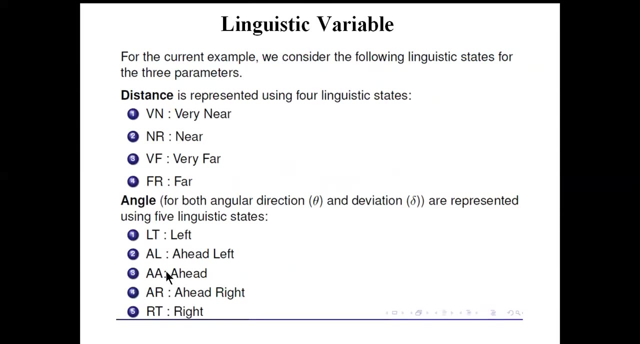 range from minus 90 degree to 90 degree, and you can see that this one is the lift. what is lt left: okay, this one is the ahead left. this one is the ahead like this: okay, sorry, so you can see that when the value is 90 degree, the corresponding membership value. 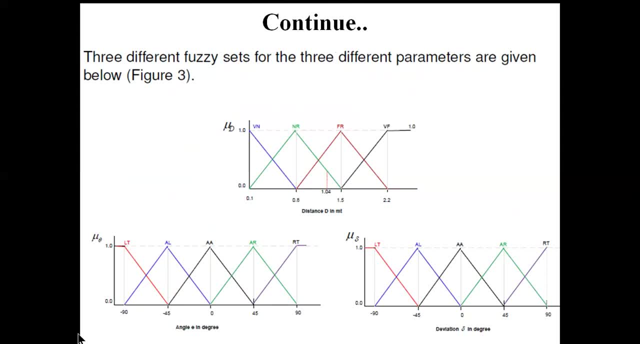 of lt is one okay when the angle is minus 45 degree. membership value function for the al is one when the angle is zero. you see it is value of a is one okay, like this way it has been defined. at the same, though, same way the deviation, or delta, is defined. 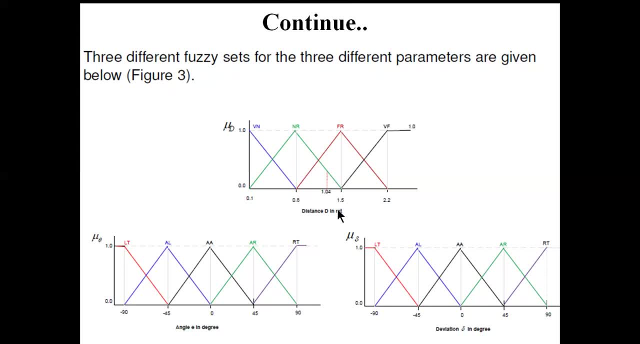 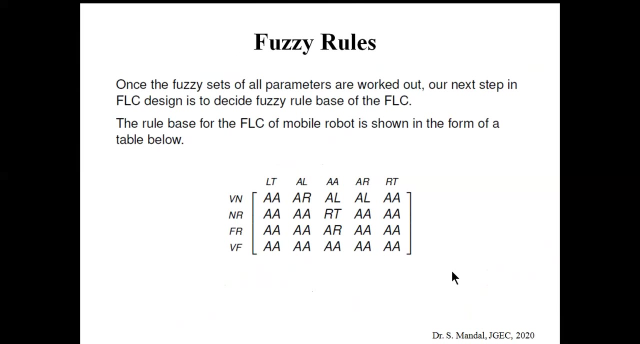 okay for the output. so this one is the distance, this one theta is the angle between the object and the robot and delta is the output. that is the deviation. delta in angle- okay, or the delta in degree, sorry. coming to the next fuzzy rules, okay. next in the fuzzy inference system there. 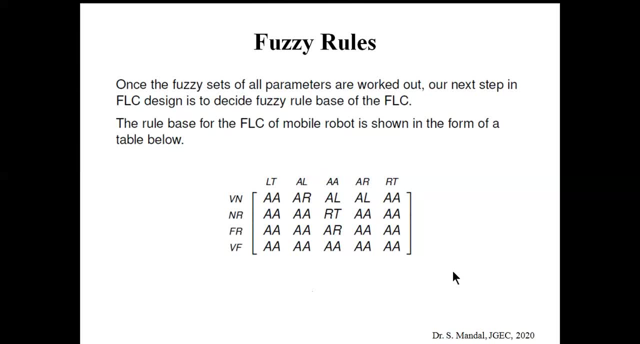 should be some kind of rules that should be defined like this: okay, so you can see that the volumes are there and we can see that when we also define, like that, this one, okay, from left, from right, second, like that, this one is going to be all the way, tw Redefinition and so on. so 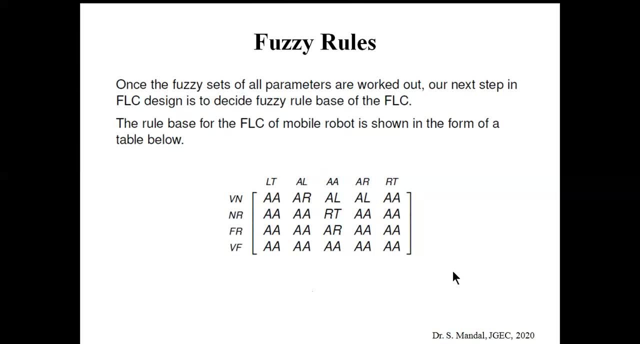 once that is already planned, we can go on to the next step. we shall go through values which are also floating here. okay, all those psychologists- he also noted that today- we, in term of, like this type of matrix, which is also known as the fuzzy rules. okay, so what is this? 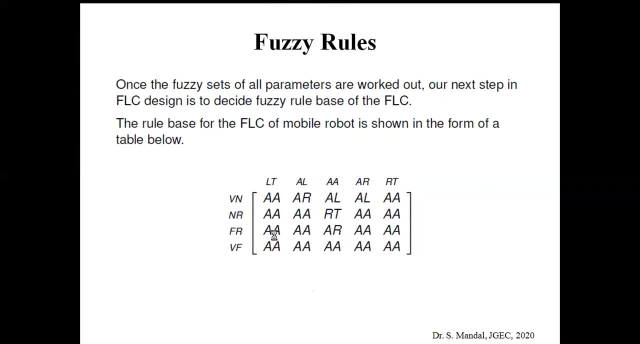 denote. basically, you can see that for this matrix or cartesian product, or fuzzy rules, along horizontal axis different linguistic state of angle are described, whereas along the vertical or along the column, different linguistic state for the distance is mentioned. okay, so this one is the angle, this one is the distance and, based on the distance and angle, the corresponding delta. 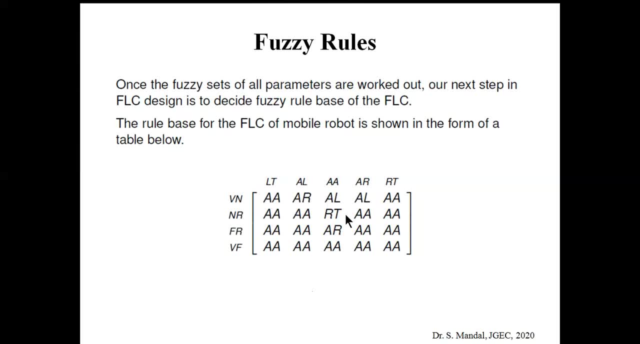 value can take either a AR, L or L. okay, so this along horizontal or row five linguistic state and on along column linguistic state for distance is described. so total: here four rule are described. how can I describe this rule? so consider the first case, row one and column one, okay, so if LT equal to, sorry, if 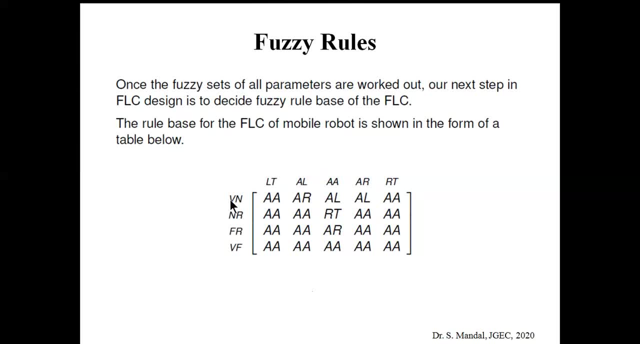 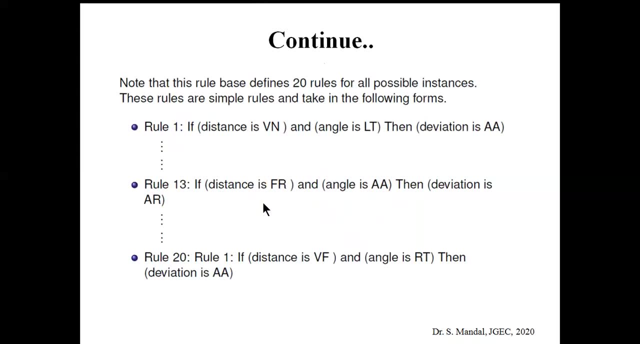 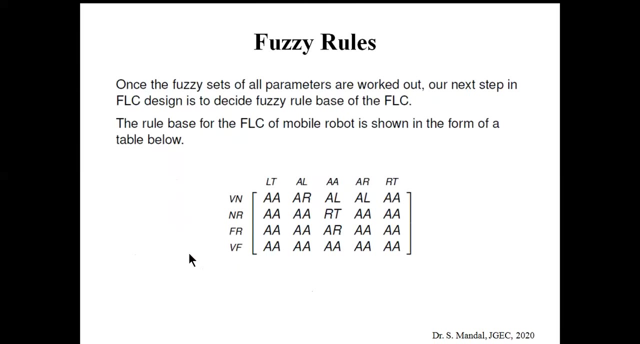 angle is LT and if distance is very near, then obviously output Delta will be AA, okay, or ahead. you can see that if distance is very near and angle is LT, then deviation is a like this: okay, now like this, one, rule number 20, or row 4, column 5, so if V, 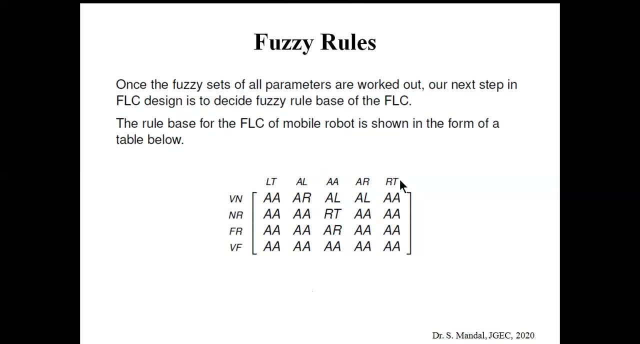 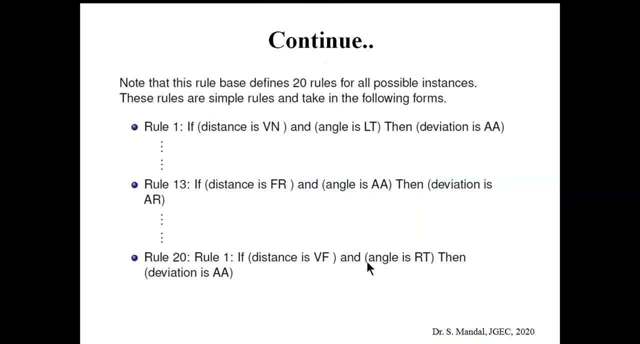 the distance is very far and angle is RT, that means the deviation will be a: a. if distance V, a band angle is RT, then the deviation is like this: this one are the for 20 different rule, 5 into 4. that means 20 different rules can be expressed. 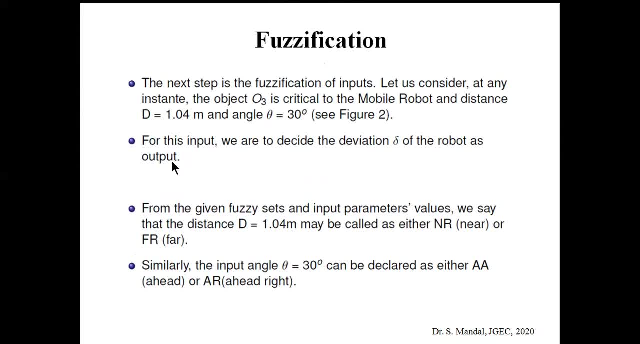 by using this matrix. now, important part of the fuzzy inferences fuzzy inference system is the falsification. that means we want to convert the input input crisp value into the falsified output. so you can see that the next step is the falsification of input. so let us consider at any instant the object. 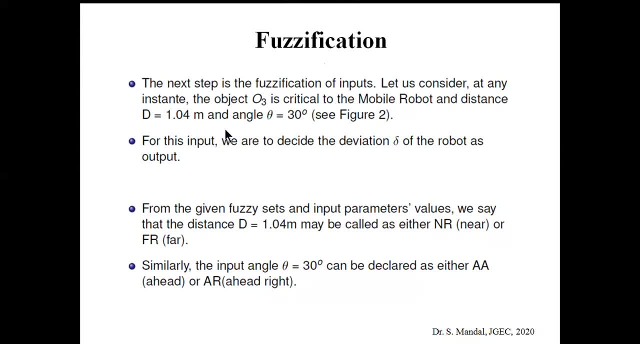 o3 is critical to the mobile robot and the distance is, like d equal to 1.04, and angle is theta equal to 30 degree. okay, now for this particular condition, or the, for the particular input combination of del, D and theta, we need to get the value. 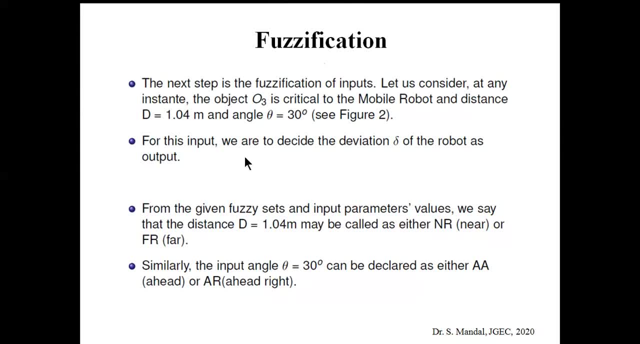 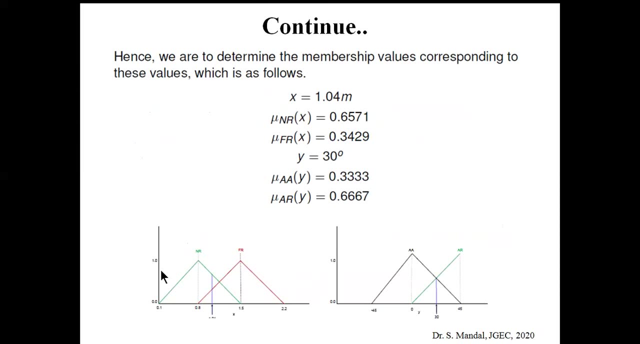 of deviation for the robot. okay, so we can see that from the given fuzzy set, the of input parameters, we can say that the distance may be called as either near or far. how can we say that that this one is the corresponding membership function of the linguistic variable? sorry of the for. 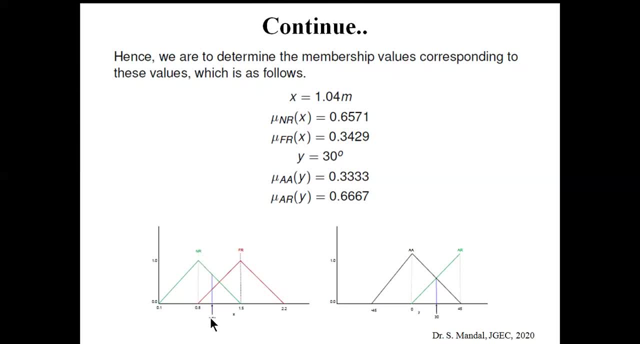 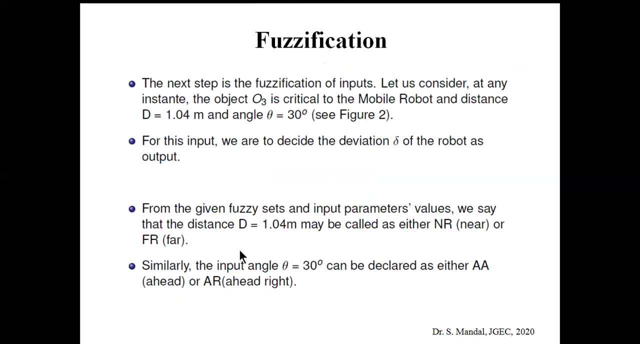 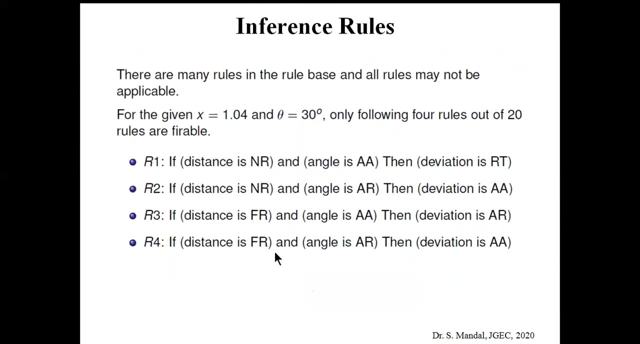 the distance. okay, so if this is the corresponding 1.04 meter, so it can touch the membership function of NR and FR only. so that's why you can say that, that the distance 1.04 may be called either nr or, far as it does not cross the others, membership. 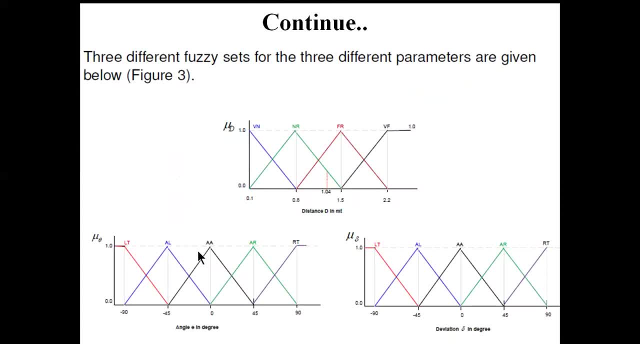 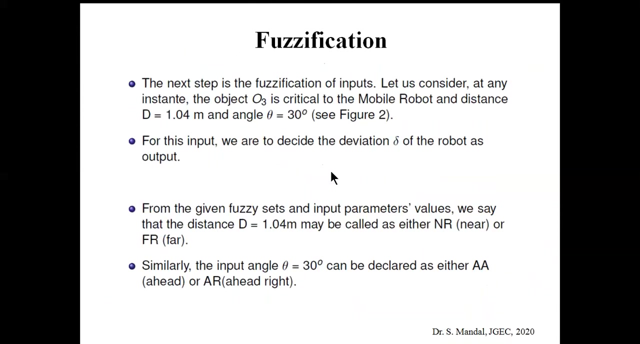 function of like this one, like, yeah, like vn or vf, this one. you can see that this one is the 1.04. so if we draw a vertical line, so it can cross nr or fr, but it does not cross vf or vn. okay, so so you only cross these two. membership function of nr and FR. similar way for the angle, theta degree. 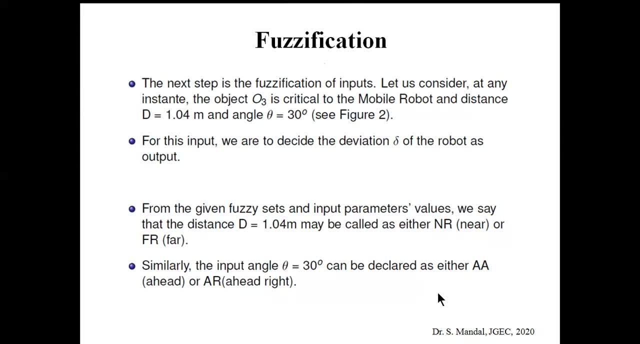 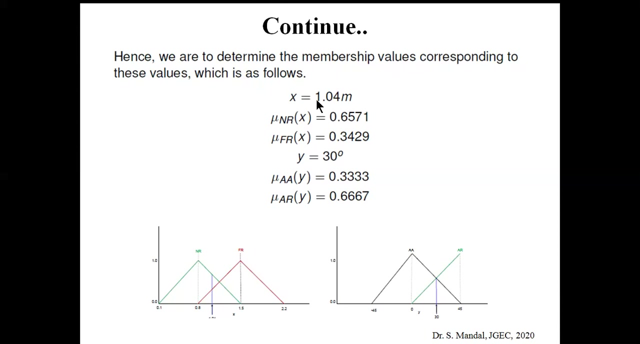 it is either ahead a or ahead right a are, because it's only cross the membership function corresponding to the a and a are. so as it does not cross the others membership function, so we need no need to bother about the otherーレ others membership value. so here you can see that for x, 1.04 meter mu membership value for the near. 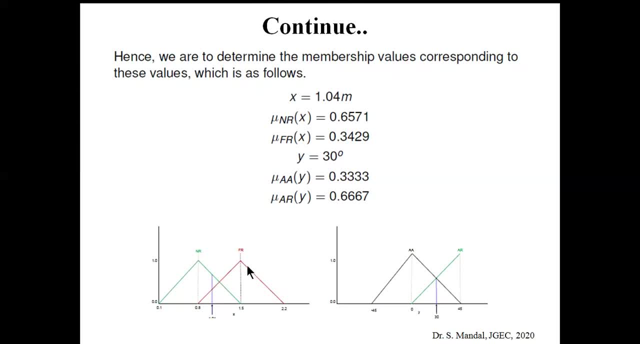 is 0.6571, from this graph we can easily get, so you can just draw it, so you can get the corresponding value from the particle. so this one is 0.6571 and for fr, you can say that this point, this or this point will be 0.3429. okay, so for, similarly, for y, equal to 30 degree, for the angle. 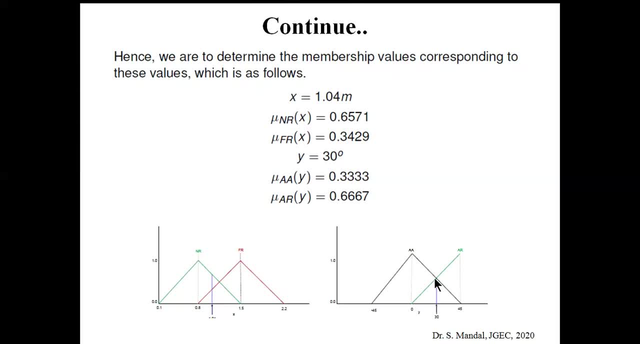 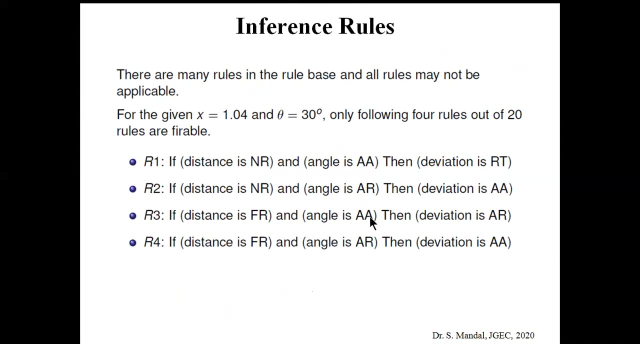 30 degree. for A, this one is 0.33 and for A R, this one is the 0.6667. okay now as x- sorry- d equal to 1.04 and theta 0.. equal to 30 degree, only touch near and a or fr and a. so we should consider only: 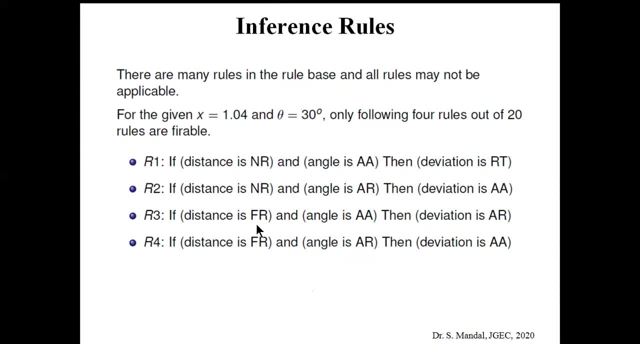 rules. those admin consists consists of, in our fr, and a air. so among the 20 rules, only four number of rules are fireable. that consists of nr, nr, fr, fr or a air, a air. okay, so we should only consider these four rules. so the rules are like this: that can be extracted from the fuzzy rule. 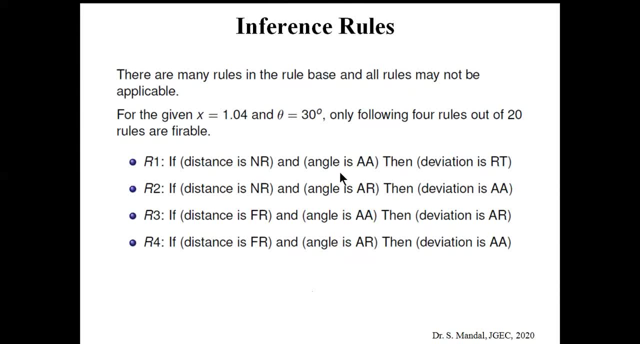 which first rule: if distance is near NR and angle is a- a, then division is RT. if distance is in our angle is a, are then the B's and its a a, and if distance is a far angle is a, then is AR. and the fourth rule: if distance is FR and the angle is AR, then the deviation is AA. okay, so 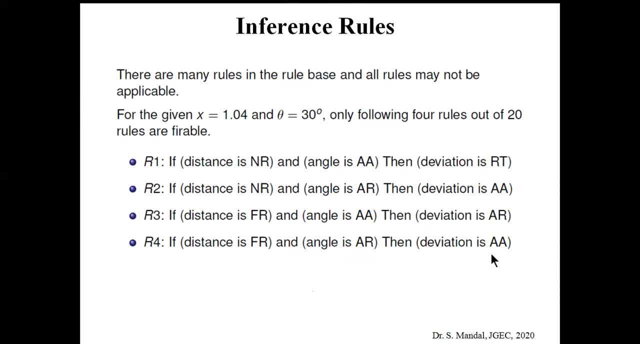 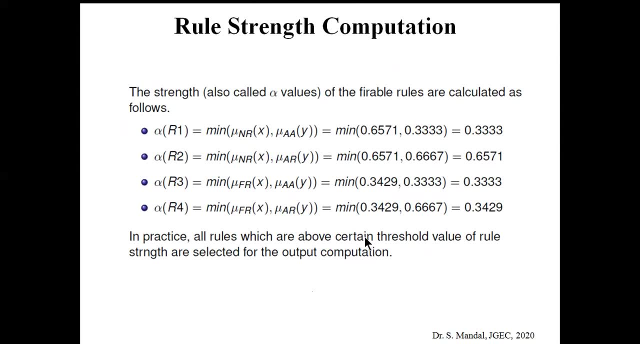 these are the four inference rule that can be used for the inference purpose. now, next step is the calculation of the rule strength. okay, so the strength of the rule- that is also called the alpha value, that is, that can be calculated by using this following formula: so alpha r1 is: 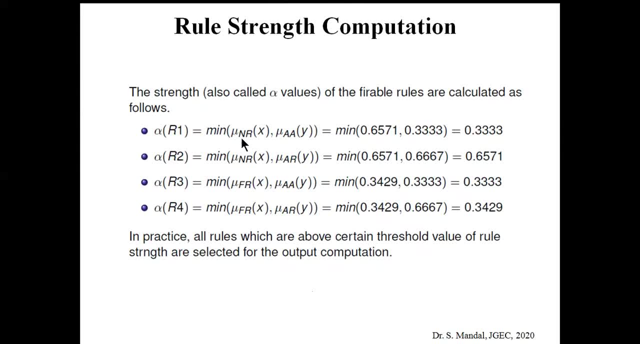 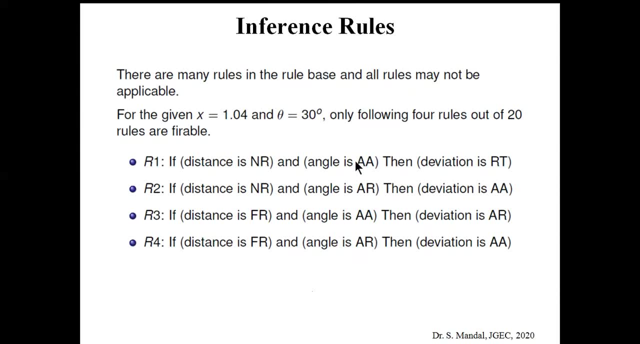 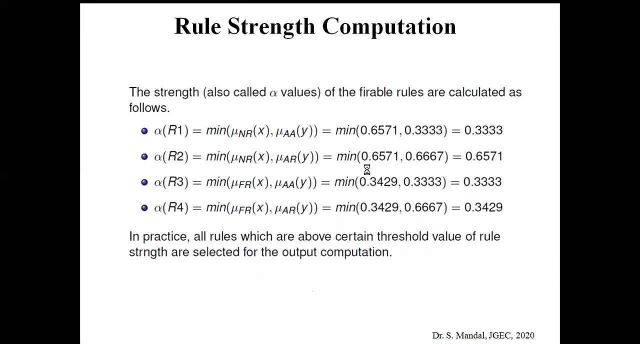 nothing but minimum of mu nrx comma mu ay. so here you can see that nr a, so the corresponding membership value for nr and corresponding membership value a. the minimum value of them is the corresponding value of the strength or alpha. So alpha of r1 is minimum of point six, five, seven, one comma, point three, three, three. so that is. 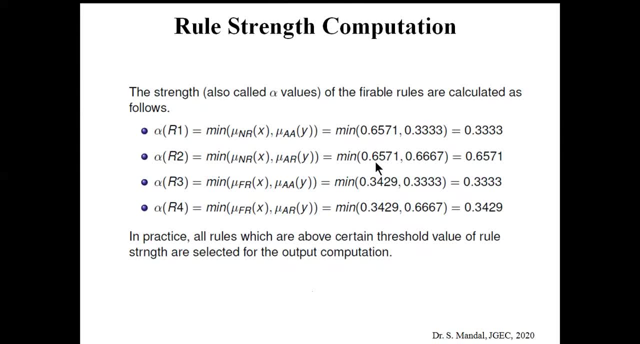 nothing but point three, three, three. similarly, alpha r2 will be minimum of point six, five, seven, one comma. point six, six, six, seven. that is point six, five, seven, one. you can see that here first of all mini mean operation or mean operator has been used. that is nothing but and operation okay. 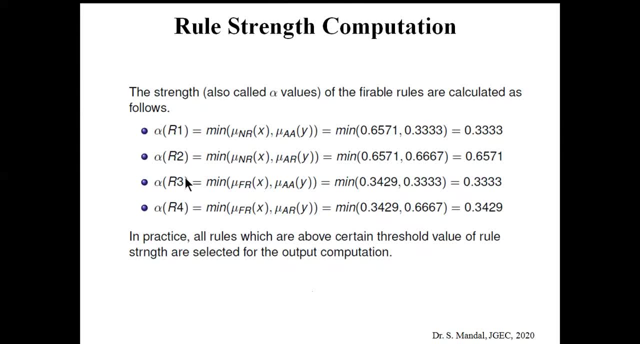 so we already told them: Mamdani process, mean function, mean max or max mean process has been used. so here you can see that. You can see that mean mean is used. okay, so in practice all rules which are above certain threshold value of rules strength are selected for the output of the competition. so forget about it. 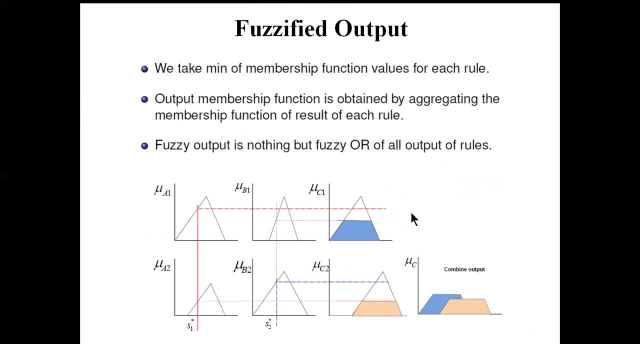 so next step will be the fuzzified output. so what it basically? the strength, what is it basically denote? so to understand that the strength is nothing: denote basically the fuzzified output part like this: So to get the fuzzified output from the rules, we need to follow the basically three step. first of, 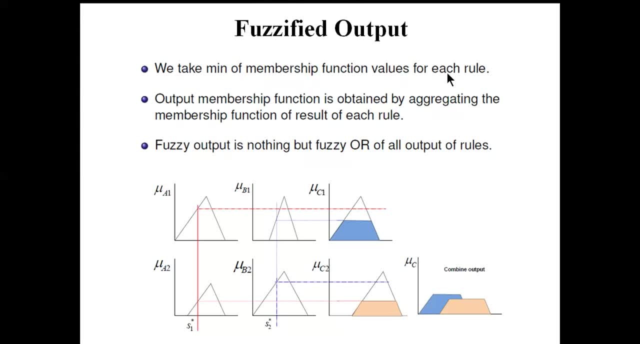 all, we take the mean value of the membership function for the each rules, so we get mean value for the each case. that is nothing but the strength. so for the like for me, when and me will be to the minimum value of them, is corresponding value, like this one. so we consider this area and similarly. 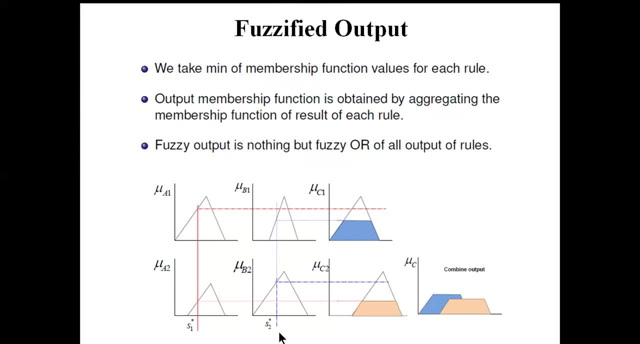 for the second rule: For the input, s1 and s2, the corresponding minimum value is like this: this one also. we consider this orange highlighted area. okay now, so our membership function is obtained. output membership function is obtained by aggregating the membership function of the result of issue, so this one is the result. 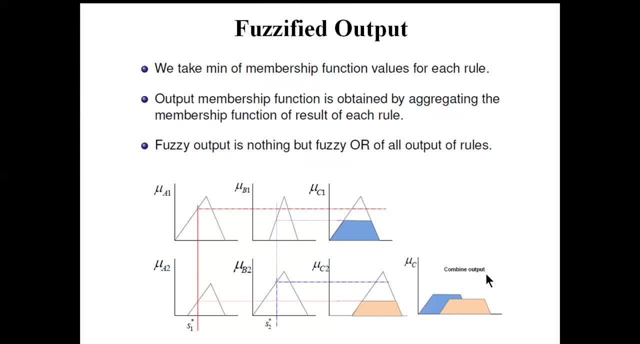 of rule one. this one is the result for rule two, so combined output for these two rules will be the fuzzy or operation of these rules. so just we need to use or operation or max operation of mu c1 and mu c2. so this is basically a simple example how to get the fuzzified output. of course, this one. 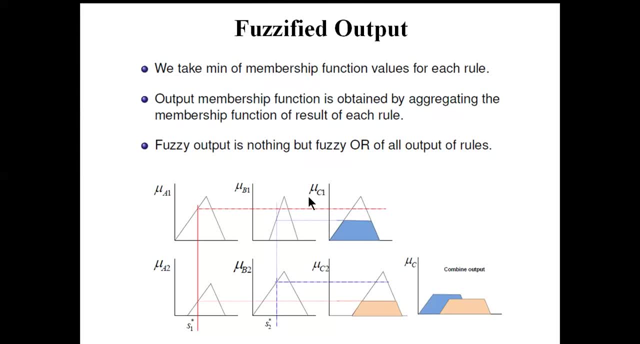 is a typical case. a, b, c are the linguistic variable and for the different input, s1 and h2- what will be corresponding? combined output or fuzzified outputs, and that will be nothing but this one. so initially we need to use mean function, then you need to use max function or or function. 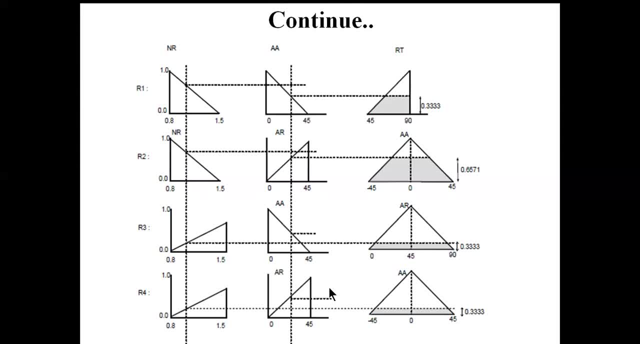 so let's now consider our particular case. so here you can see that this one is the rule one. rule two, rule three, rule four: these four rules are used for the our particular problem of mobile robot. so for particular case of nr and a, you can see that rule, rule one. what is rule one? 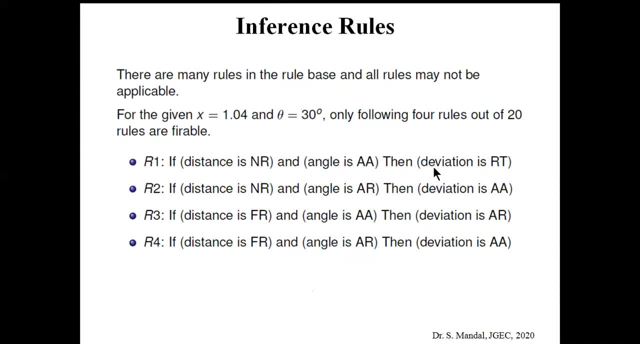 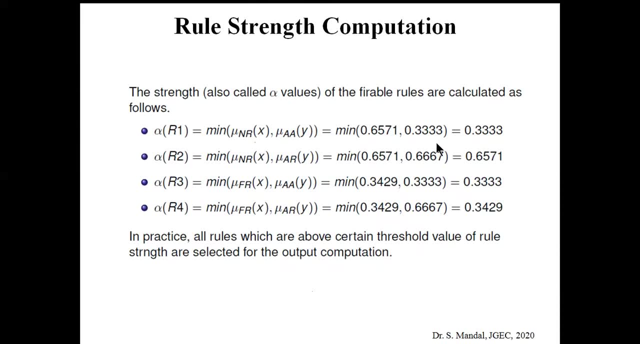 rule one is for: if distance is nr and angle is a, then deviation is rt. okay, so you can see that for nr, value is 0.6571 and a value is 0.333, so obviously, so just we use 0.6571, and this is one. 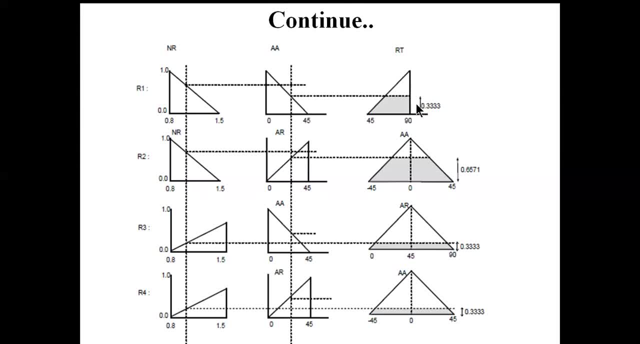 point three. three, but the minimum values. we should consider 0.33. so we should consider the area of rt, this area, so this one is the a1. okay. similarly, for rule two, we should consider the minimum minimum value, that is, 0.6671. the height, height of the membership function. so this is. 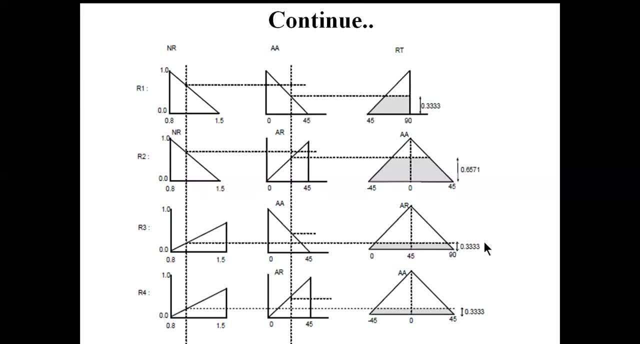 basically this value- 0.6671 for the rule, or rule 3, 0.333, and similarly for rule 4, 0.333. all these denote the strength of the corresponding rules. that means minimum value of the different input combinations. okay, so this one is the d, equal to 1.04. this one is the theta, equal 30 degree, and. 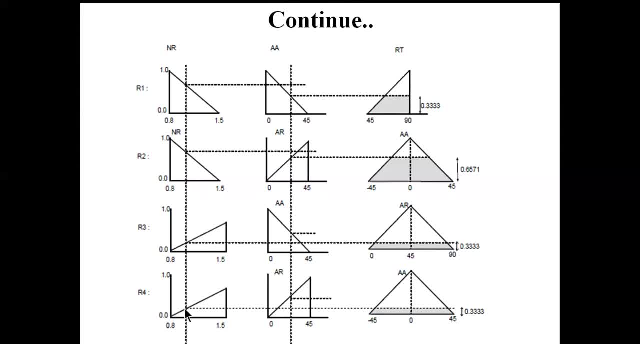 you can see that for different value of rt, this one is the theta equal 30 degree. and you can see that for different value of rt, this one is the theta equal 30 degree. and you can see that, for different value of rt d and theta and corresponding 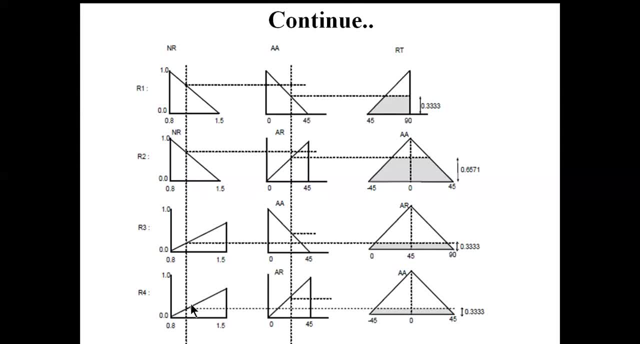 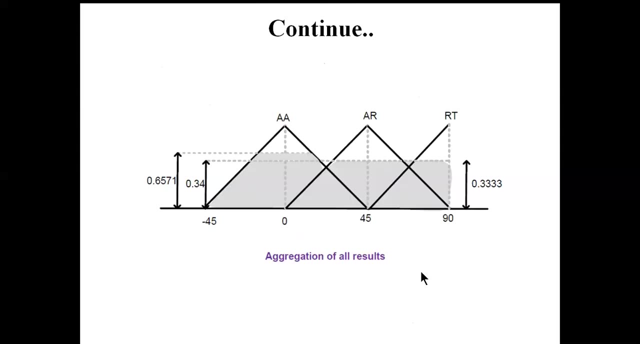 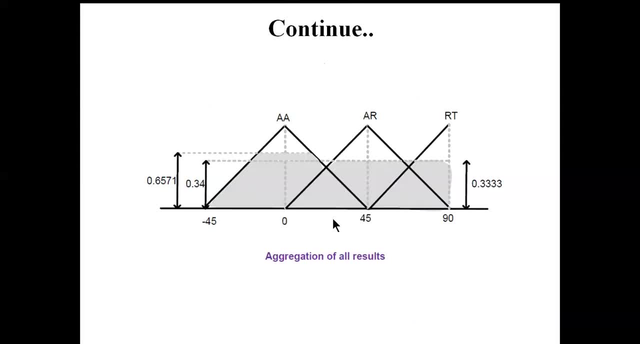 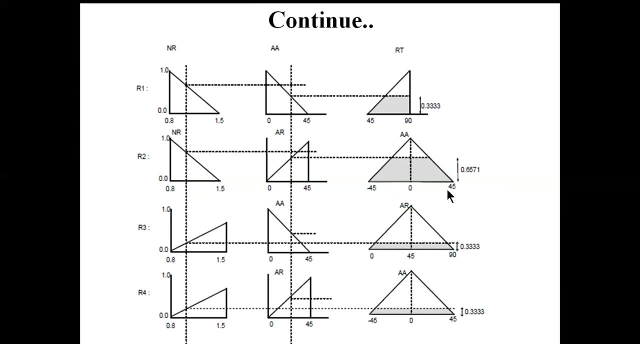 maximum value is 90 degree. so obviously the fuzzified output will be from minus 45 to 90 degree and if we add them, that means if we take the maximum value from minus 45 to 45 degree. maximum value- sorry, maximum value of the membership function. 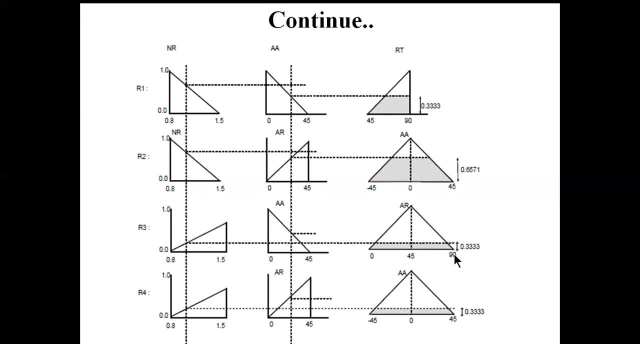 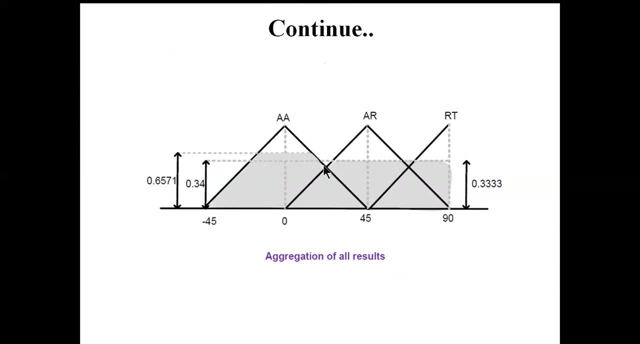 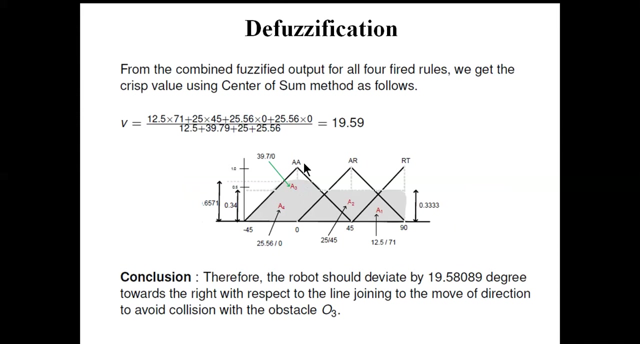 in the range of minus 45 degree to 90 degree. so the corresponding fuzzified output will look like this: this one, this, this, this, this. okay, so this one is the fuzzified output. so this one is the fuzzified output. so this is the fuzzified output. 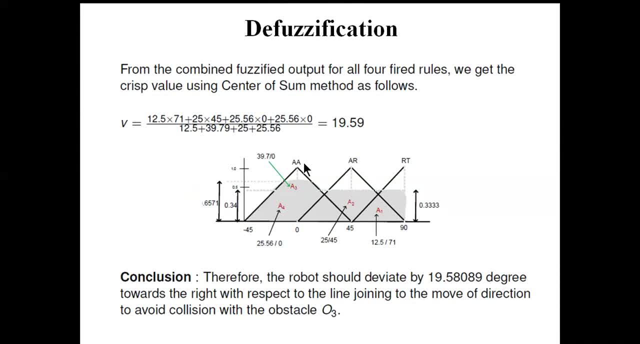 and then, um, we can get this by using fudgy or mamdani inference method. now, next process is the defazification. so obviously, uh, to use, or to use the, or to get the output in real life that should be in the crisp value. okay, so to get the crisp value from the diff, from the fuzzified output we need to use. 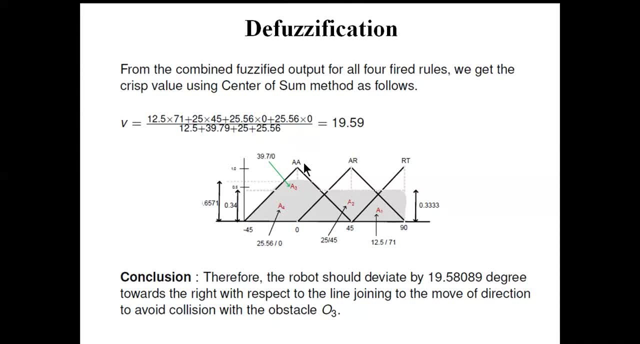 so to get the crisp value from the diff, from the fuzzified output, we need to use some kind of defazification technique here. we can use, or we have used, center of some method. so that is give given by the crease output as summation of X- I. 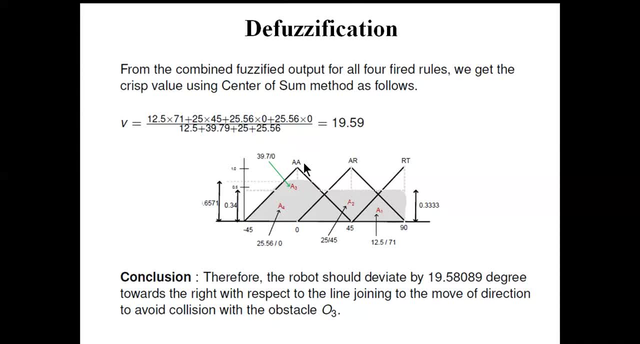 into AI divided by summation of AI, okay, where X, I is the geometric center and AI is the corresponding area of that portion. so here there are four numbers of area: a1, a2, a3 and a4. so the area of the a1 is 12.5 and a2 is 25. it a3 is 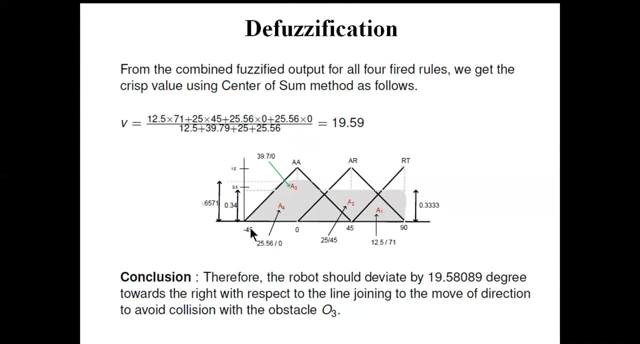 39.7 and for the a4 is 25.56. that can be calculated using simple geometric process. okay, now we need to identify the XI. that is nothing but the geometric center. so for the geometric center of a1 is the 71 degree. for for the geometric center of a1 is the 71 degree. 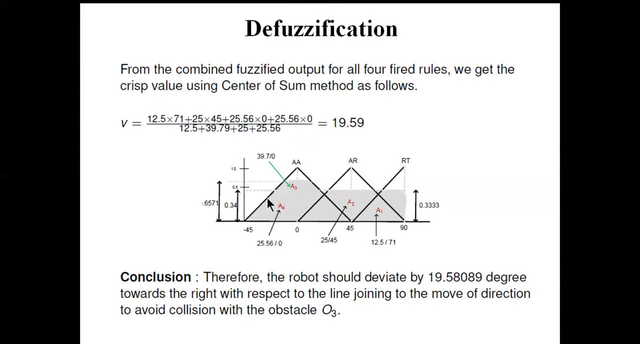 for a2, 45 degree. for a3, a3, you can see that a3 for this area, so you can see the geometric center- is 0, so here it is 0. and for a4, similarly, this area, that is also 0. so by using the simple formula, 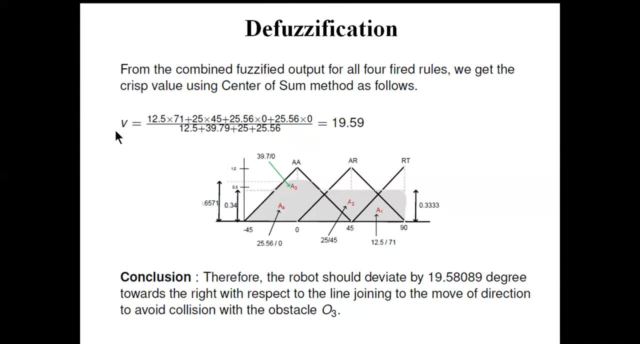 of cos method we can guess the crisp value of delta, that is 12.5 into 71, 25 into plus, 25 into 45, plus 25.56 into 0 plus 39.7 into 0. sorry, this one been repeatedly written. that should be 39.7. 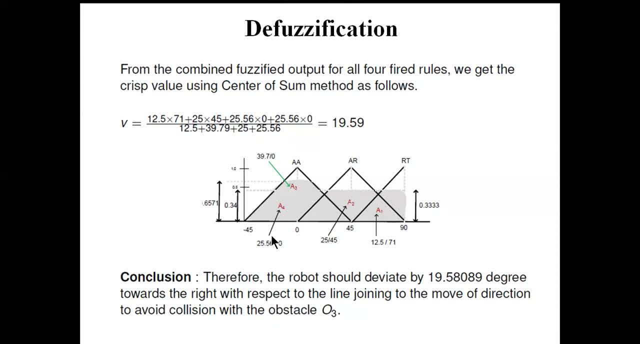 okay, so and and denometer will be area of them, summation of area of them. so 12.5 plus 39.7 plus 25 plus 25.56, like this way, okay, and the corresponding output value is 90.59. so therefore, the robot should. 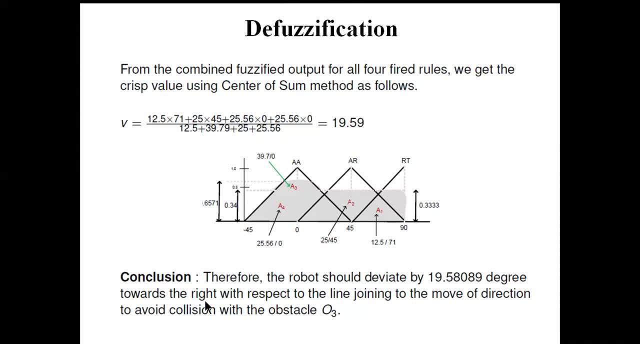 deviate 90.59 degree towards the right. towards the right, with respect to the line joining to, to respect to the line joining of the move of the direction, to avoid collision with obstacle o3. okay, so like this, so you can see that without using any mathematical formula or without using different any.